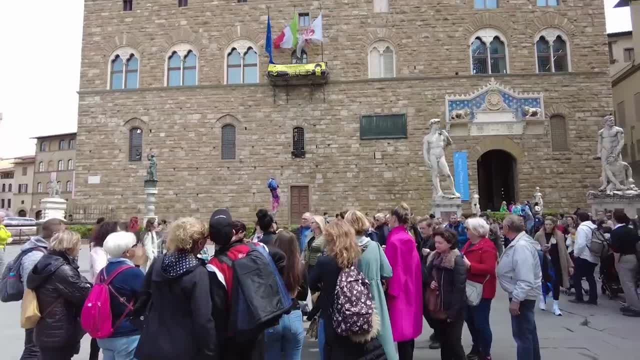 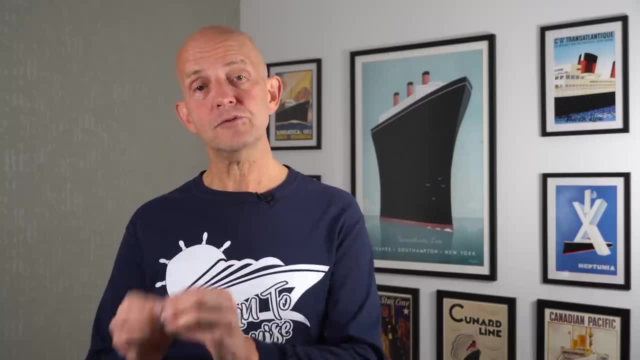 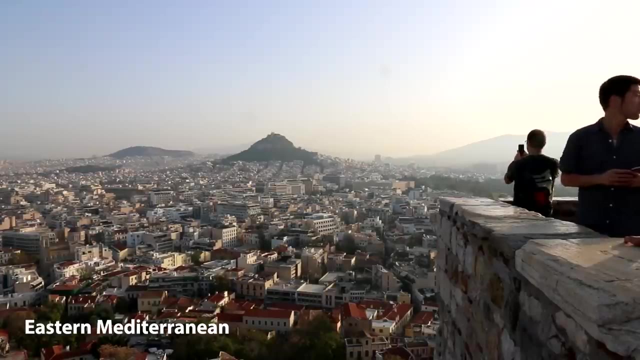 museums, architecture, culinary and wineries. I suggested to Winnie that if she enjoyed a Western Mediterranean itinerary and wanted to go on another one, her next should be an Eastern Mediterranean one. This is probably my personal favourite. Departing mostly from ports around Venice and Piraeus, near Athens, these visit Italy. 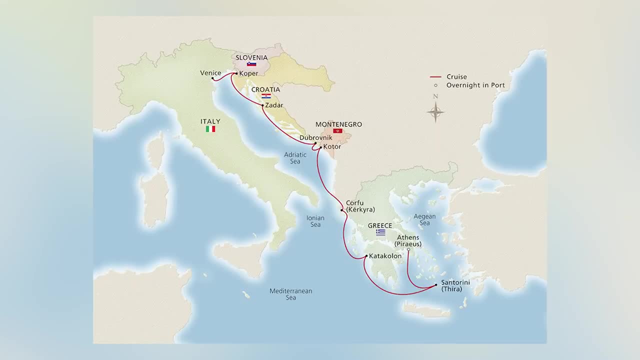 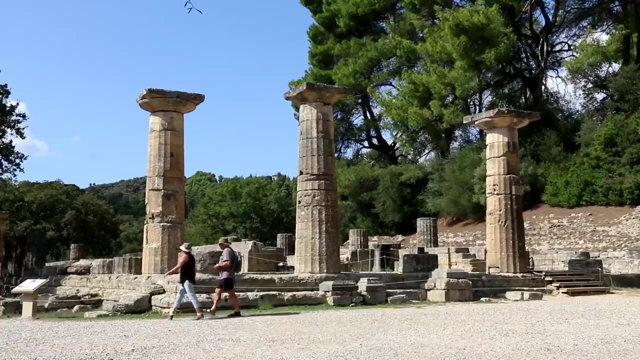 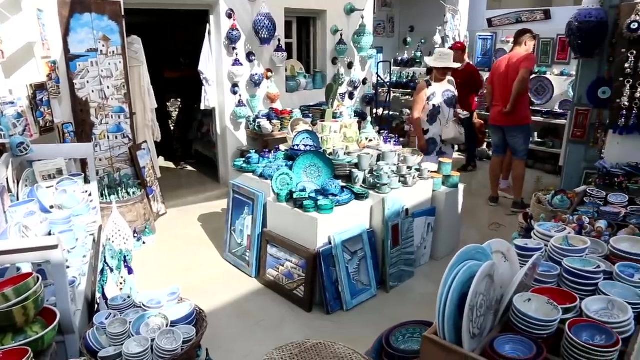 Croatia, Montenegro, Greece and sometimes even Turkey. The most popular ports include Split, Dubrovnik, Corfu and Greek islands and ports like Katakolon, Santorini and Mykonos, While the itinerary and excursions also focus on culture, historical sites, museums and architecture. 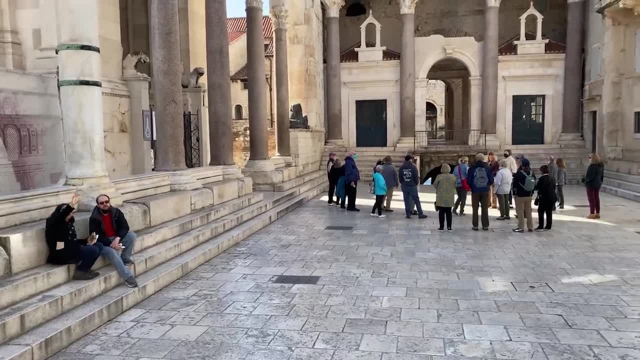 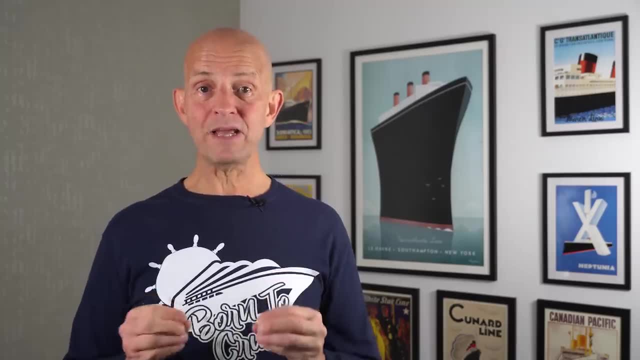 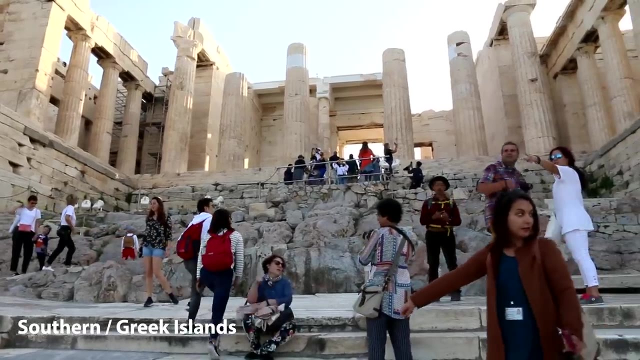 they tend to be more on the active side. I said to Winnie if she wanted to return to the Mediterranean after I recommended a more southern and Greek islands itinerary, especially if she wanted to have more of a beach mixed with ancient sites, Mostly sailing out of Piraeus near Athens. the islands visited vary based on the size of ship. 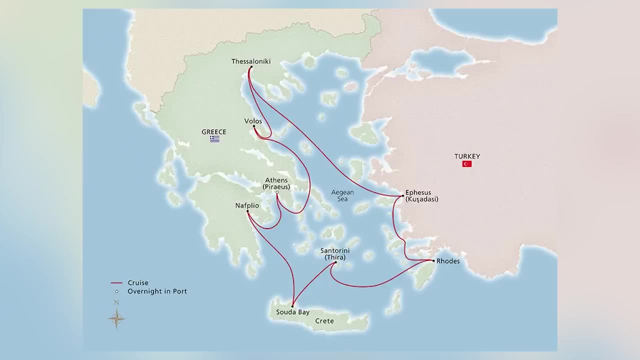 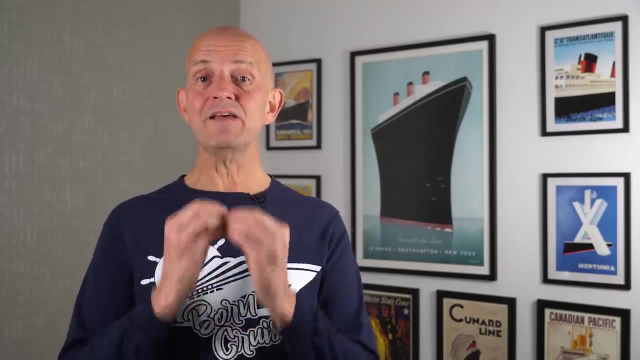 so smaller ships call on more out-of-the-way islands, as well as the large and best known ones, and Mykonos, While those three Mediterranean cruise options tend to be seven nights long, a meter away from the Mediterranean is much longer. The coastline of the island is much more. 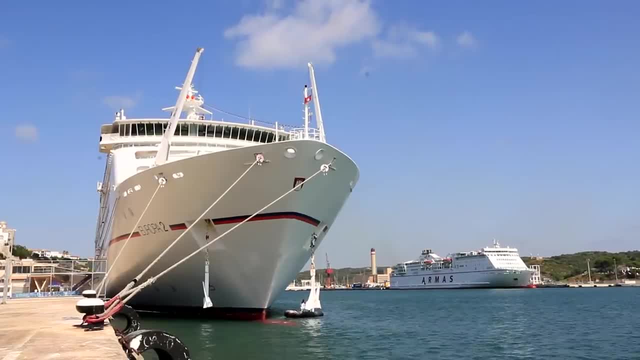 varied and the water is not very clear. As a result of increasing water content, the water has much more water to drink, and the water has much more water to drink. request for a week-long cruise. there is a big blunder that many people make, as I have. 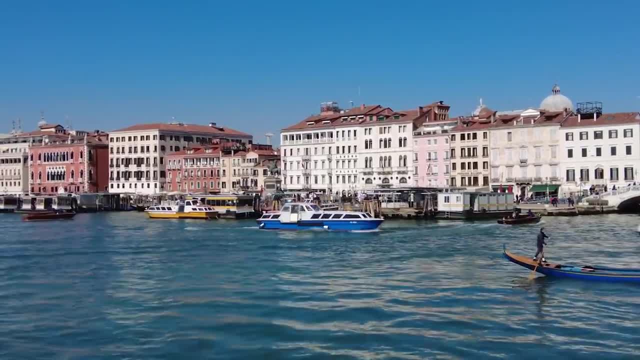 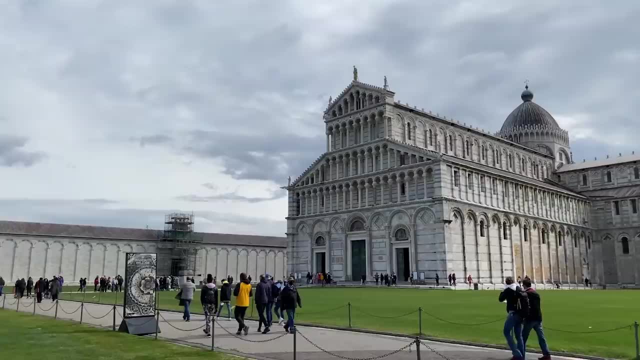 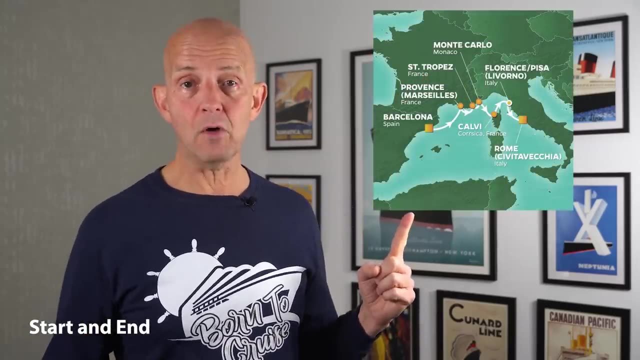 in the past that I also needed to warn her about. next, First, whatever week-long itinerary she books will always include one or two must-see cities that she thinks she will see but won't see at all. For example, I showed her the 7-night Western Mediterranean cruise. I was about to go on. 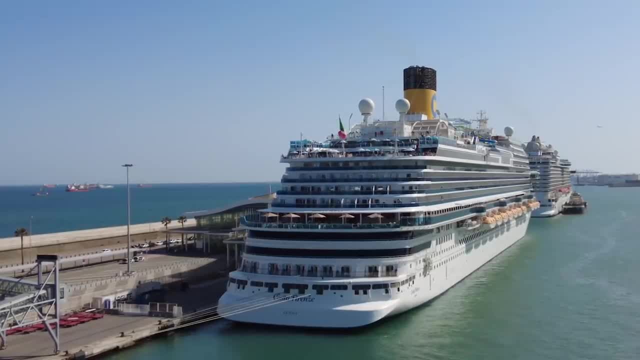 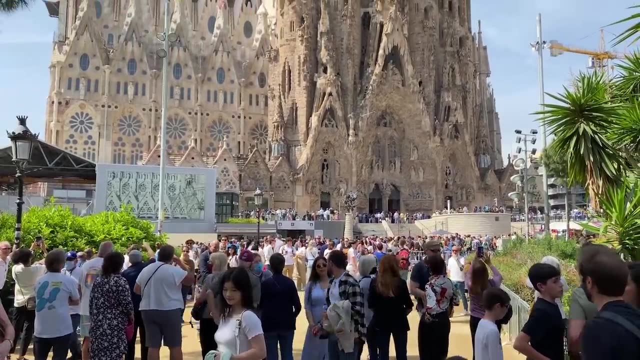 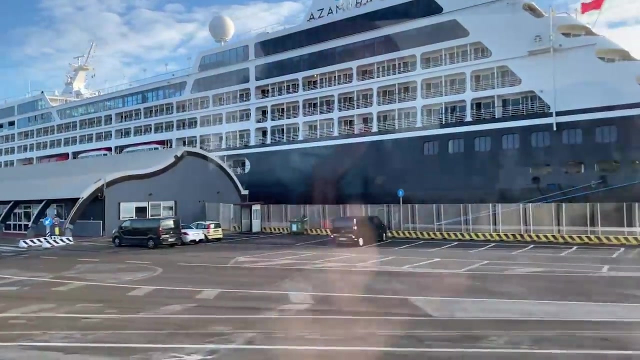 The advertised itinerary prominently calls out Barcelona and Rome as two ports, but they are where I embark and disembark. If I hadn't booked a pre-stay in Barcelona and a post-stay in Rome, I would see nothing at all of those cities, other than glimpses from the bus or taxi window while being transferred. 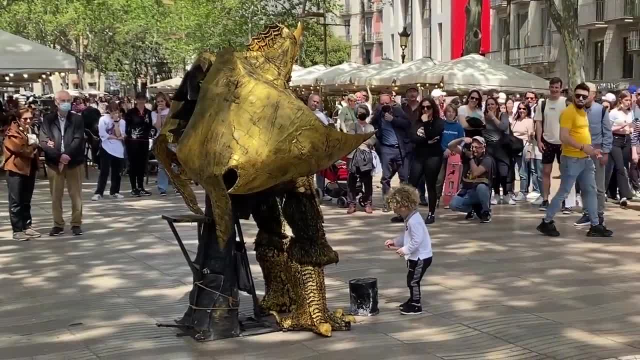 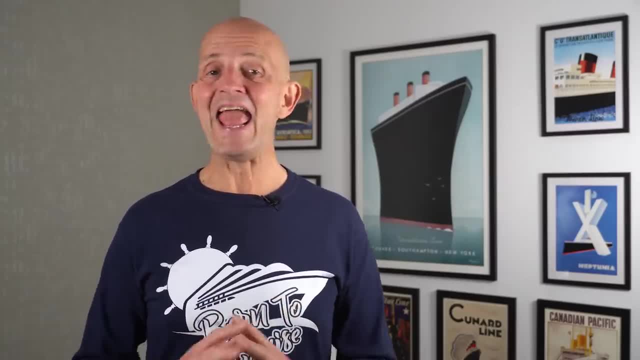 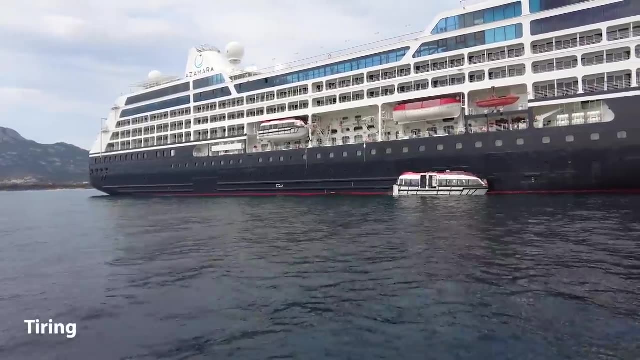 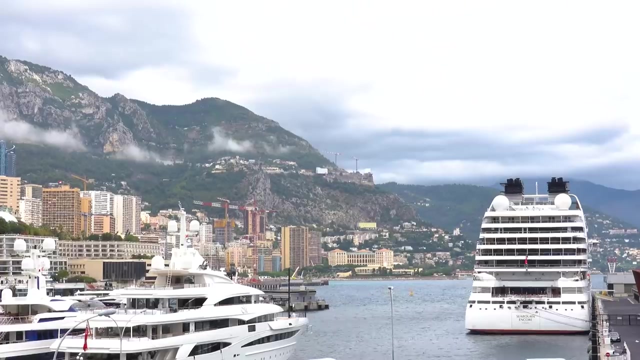 between the airport and the ship To see the cities where Winnie embarks or disembarks. I strongly encourage her that she must add stays there. Second, most underestimate how tiring a week-long Mediterranean cruise can be. If you have sea days for Winnie to relax, she will be out exploring most of the day. 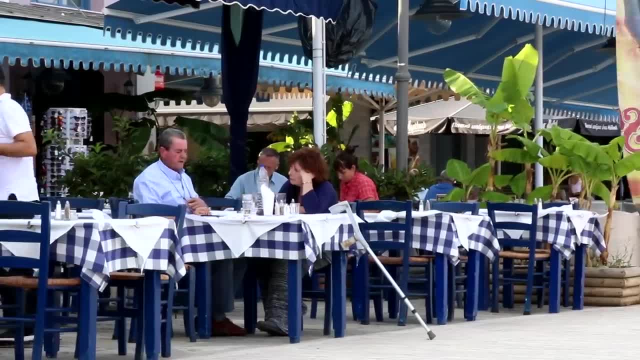 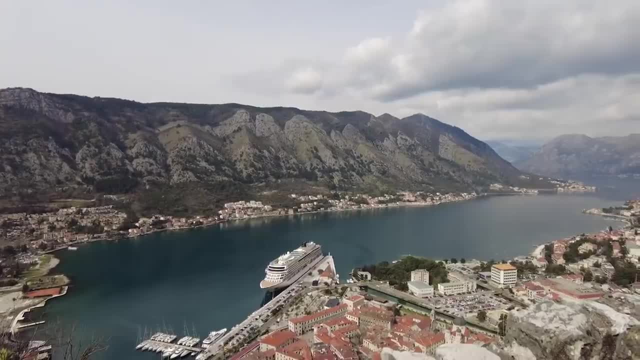 and enjoying the dining and entertainment well into the evenings. She will be flying in so likely tired and jet-lagged- another good reason for having a pre- and post-stay. And thirdly, this is all magnified as quite a few Mediterranean ports are far from the 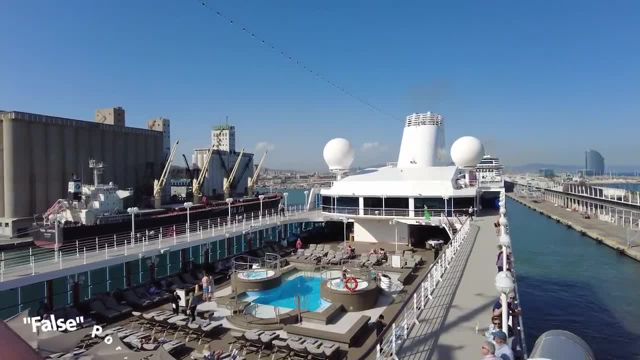 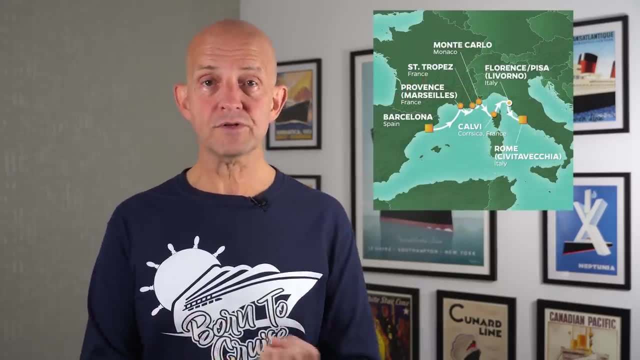 advertised city or sites, which means many of her excursions could be 8 to 10 hours long every day. Look at my upcoming cruise as an example. The itinerary is advertised as Provence, Marseille, Florence, Pisa, Livorno and Rome Cicciavecchia. 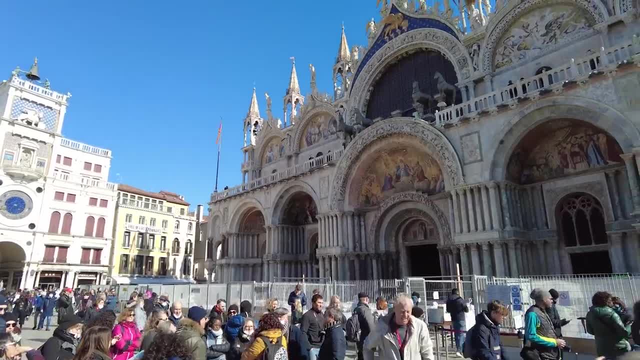 On Eastern Mediterranean ones. you might see Venice, Livorno or Trieste, Olympia, Catecholone and Piraeus, Athens. The time to get to the Mediterranean is about 8 hours. The time to get to the Mediterranean is about 8 hours. 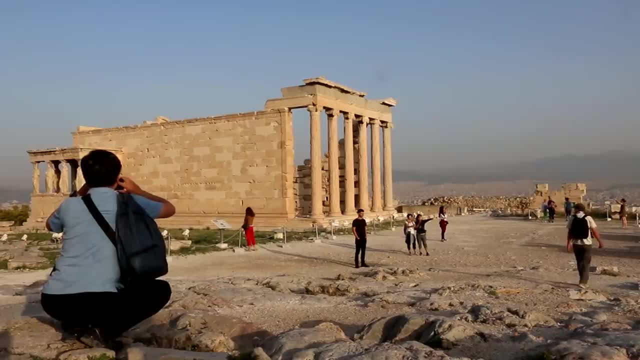 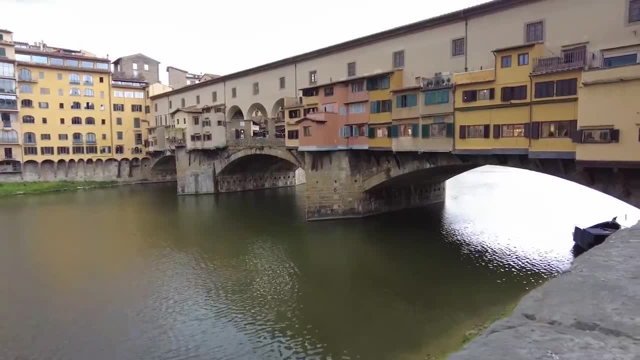 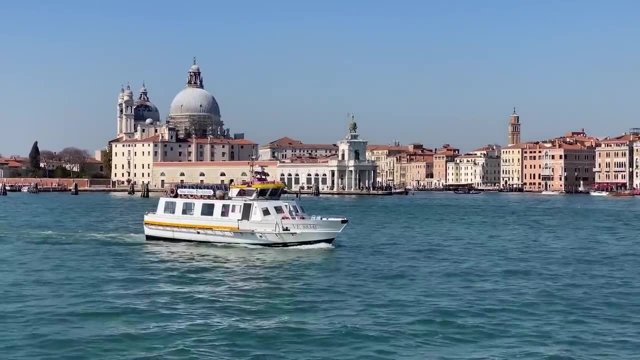 Rome can take up to 2 hours each way, based on traffic from Cyssavecchia, Florence. 1.5 to 2 hours each way from Livorno, Venice, which most ships couldn't sell anymore. used Livorno or Trieste, which was 2 hours drive away. 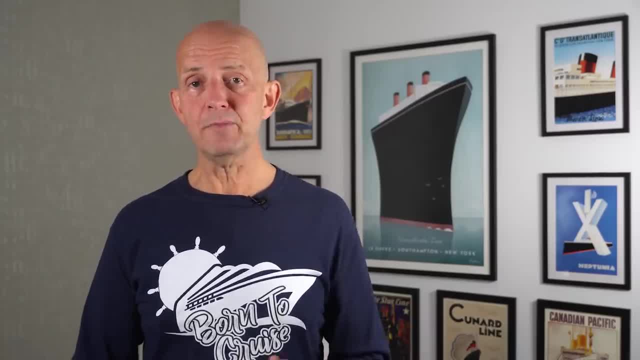 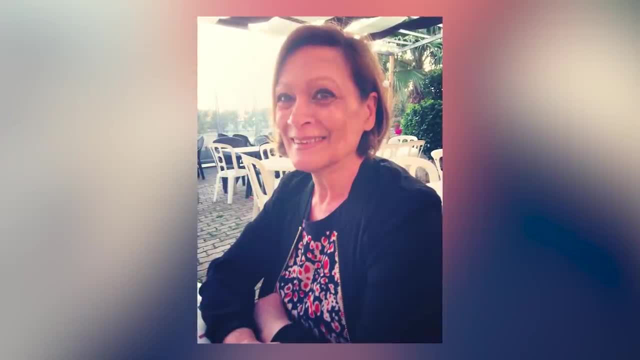 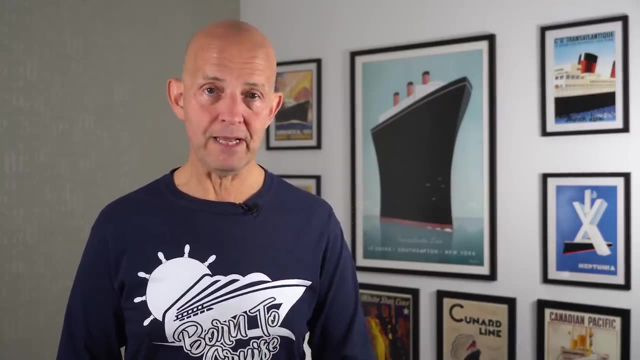 Even more. places like Olympia from Catecholone, Cicchateria from La Spezia can take up to an hour each way. With Winnie understanding the issues around week-long trips, I wanted her to now tackle her plan to cruise in July, a blunder so many people make. 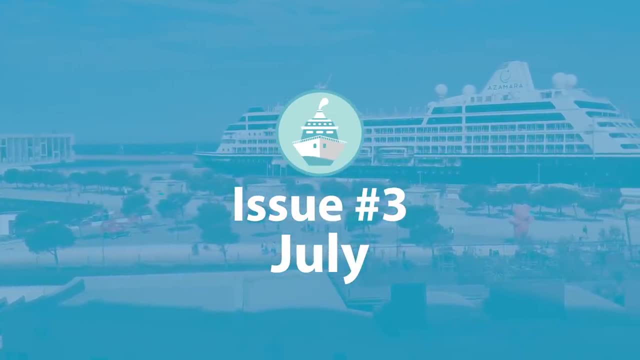 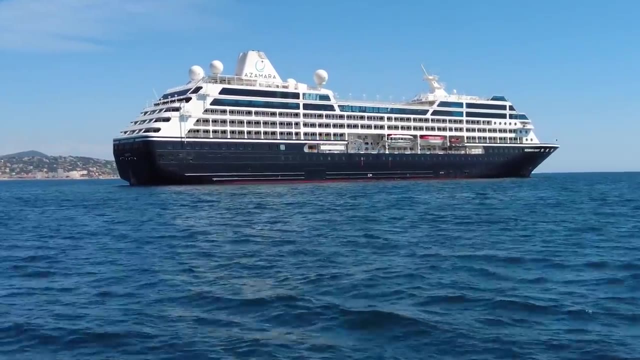 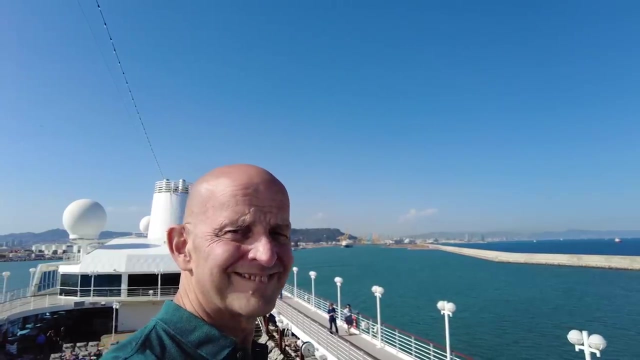 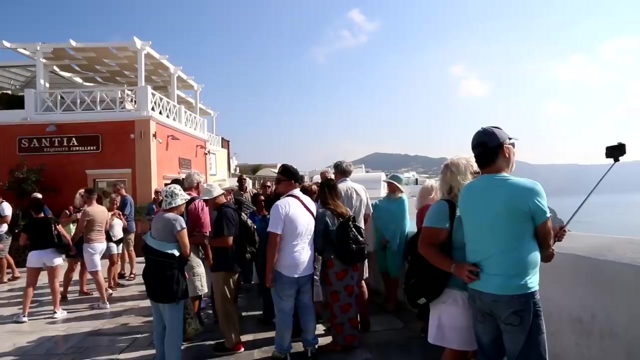 The Mediterranean cruising season runs from April to October, although a handful of ships will sail year round. I warned Winnie that going in July and August is a mistake for five key reasons. First, it gets hot and sticky very. Secondly, it is peak season and extremely busy with both cruise and land-based travellers. Some Mediterranean countries, including France, Spain and Italy, close their factories and businesses in those months and everyone goes on vacation, mostly in Europe. It is hard to get into places. there are crowds everywhere. Third, it is the most expensive time of the year to go. 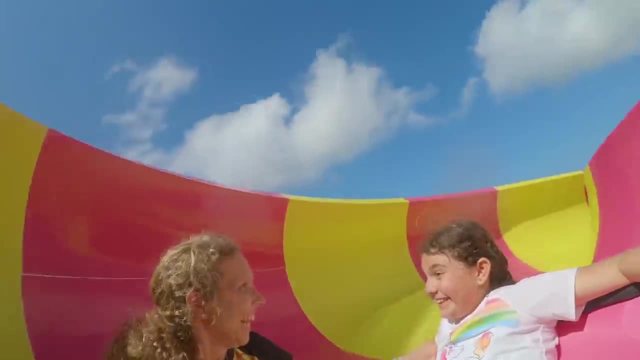 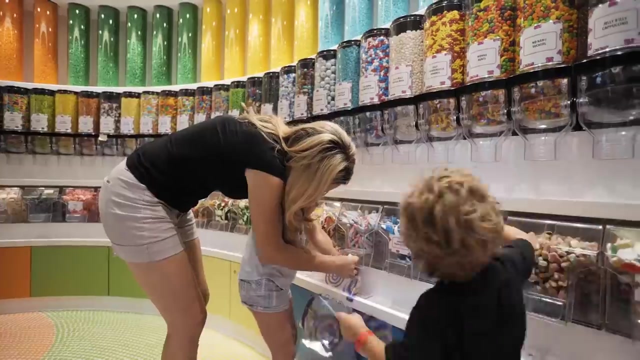 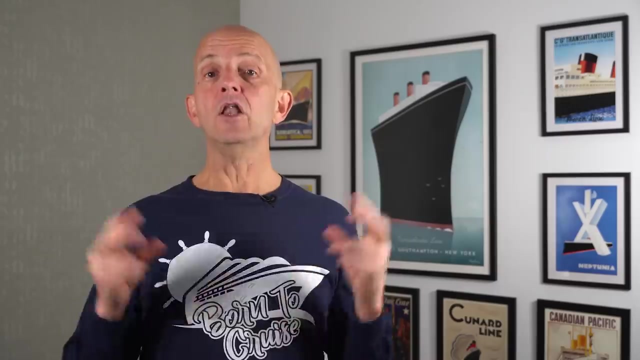 Fourth, as it is school holidays, Families will be cruising. even on lines that usually don't have kids will have kids. I told Winnie this is important because many ships will be sailing way over capacity. When ships declare occupancy, it is based on what is called lower berths, which means 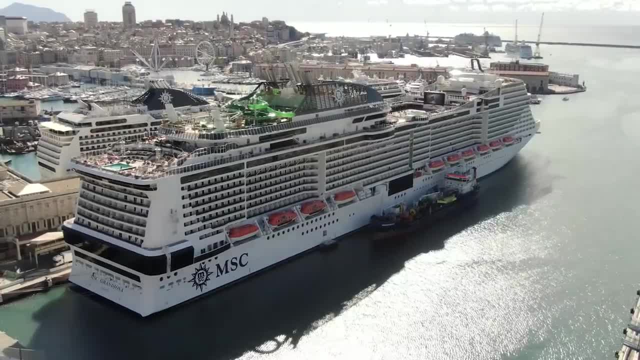 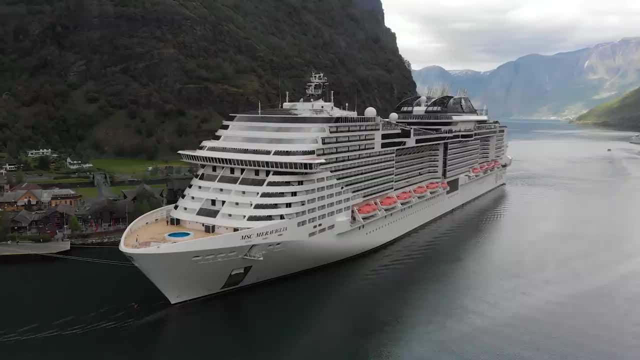 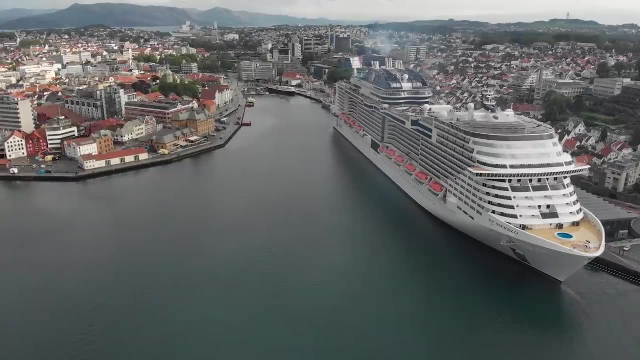 two people per cabin and doesn't count sofa beds, pull down beds and other places where people can sleep. For example, when I was on an MSC Cruises Meraviglia a couple of years back, they told me their official capacity was 4,500, but in July and August they often have 6,000 passengers. 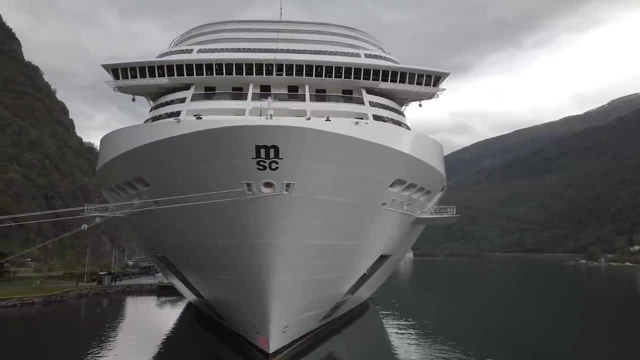 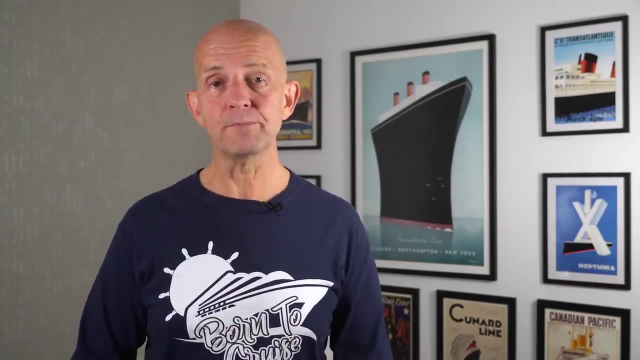 because kids are sharing cabins with their parents. While other ships may not be as dramatic as that, all are likely to be at higher capacity when families are on board. Fifth, I warned her this is the prime scam and pickpocket season, due to the peak and 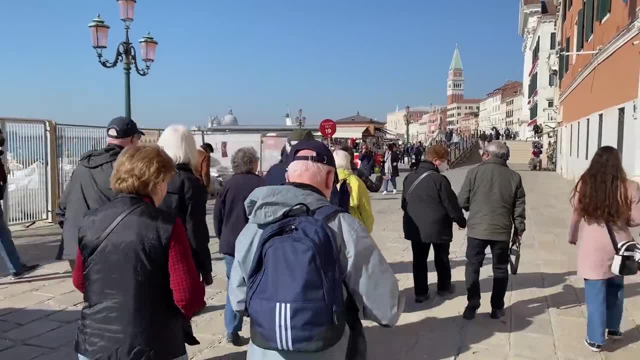 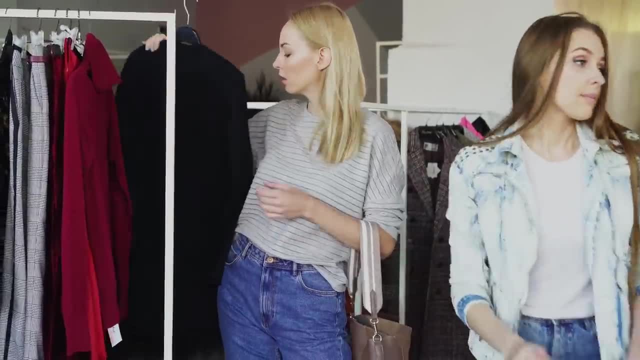 jostling crowds. To be honest with you, every time I have been in Venice, Barcelona and Rome, I have been on a cruise. In that peak July-August time. people off the ship have had wallets stolen, bags snatched and backpacks opened. 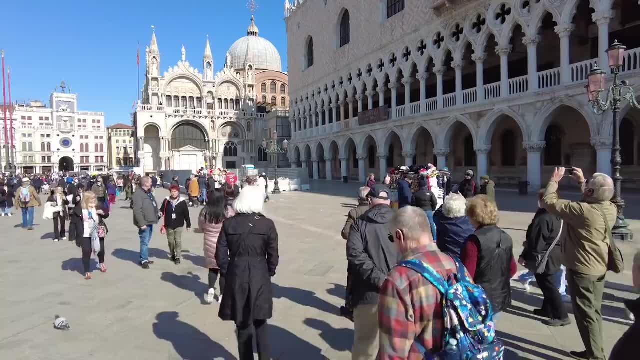 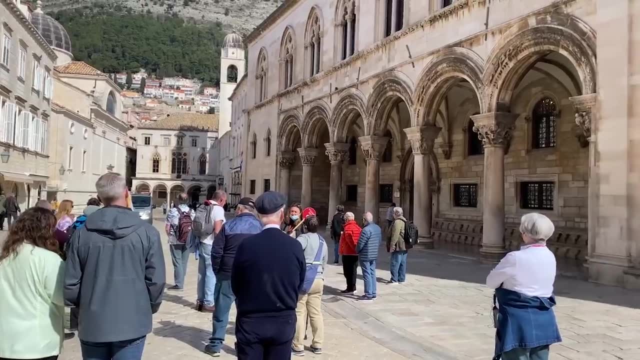 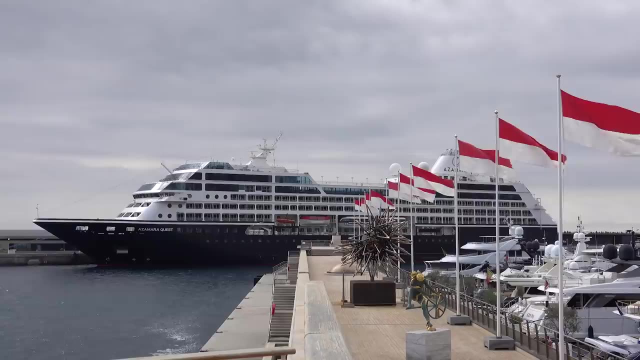 I suggested. Winnie instead looks at the shoulder season. June and September are especially great months, though May and October work as well. Everything is open, it's great but not stifling weather, and since Winnie doesn't have to go in school holiday time and is going with a friend of hers, they will have a less costly. 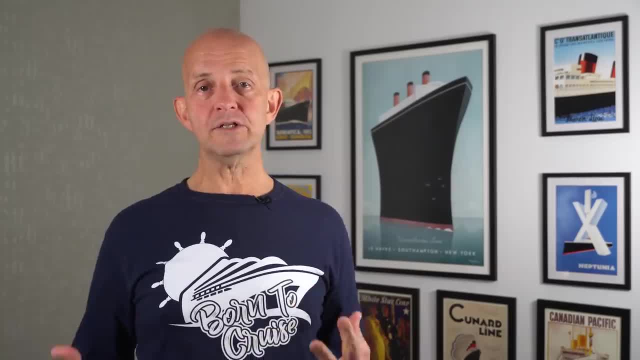 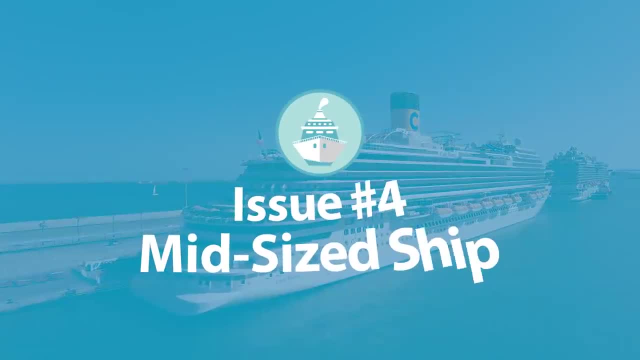 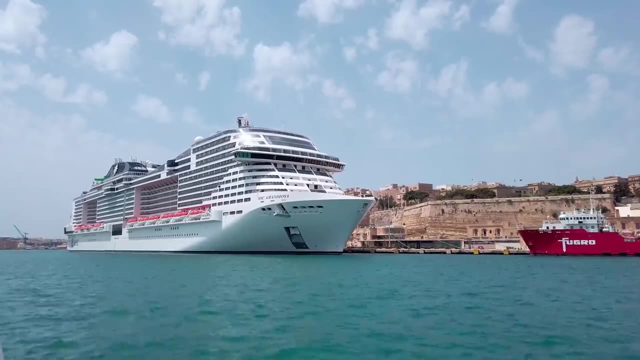 and much less crowded trip. Winnie had said that she wanted to go on a cruise, But I worried she was falling into another trap. here too, I suggested she step back, as there are a few considerations before settling on ship size- and another blunder I have seen make. There is enormous line and ship choice in the Mediterranean, so first I suggest we cut out the number of lines she should consider based on her budget. Pretty much every cruise line, ranging from the most inexpensive to the most expensive, like MSC, Norwegian, Carnival and Royal Caribbean, through to the most expensive cruise lines. 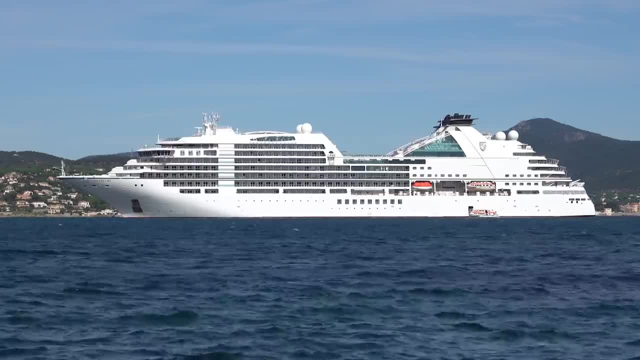 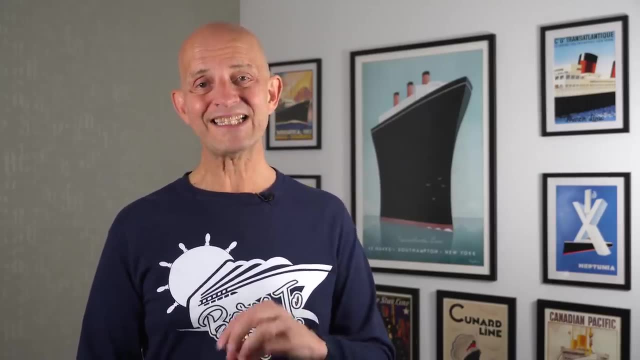 in the world, like Regent, Seven Seas, Seabourn and Silversea cruise. here They basically offer the same itineraries and ports. For example, Winnie could book a 7-night Mediterranean cruise next June for two people on MSC SeaView. 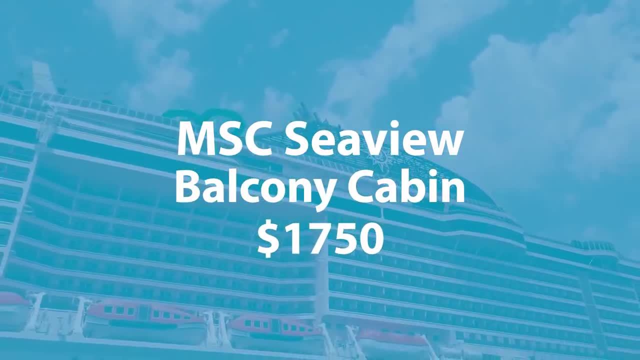 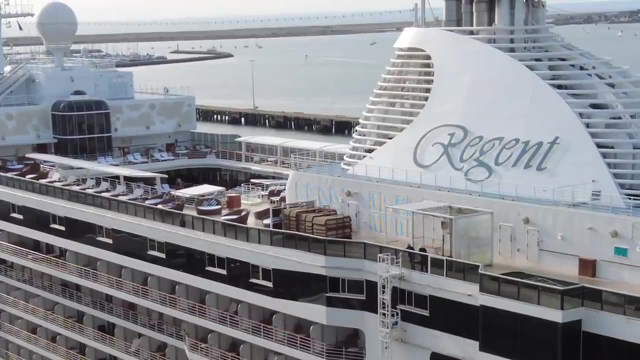 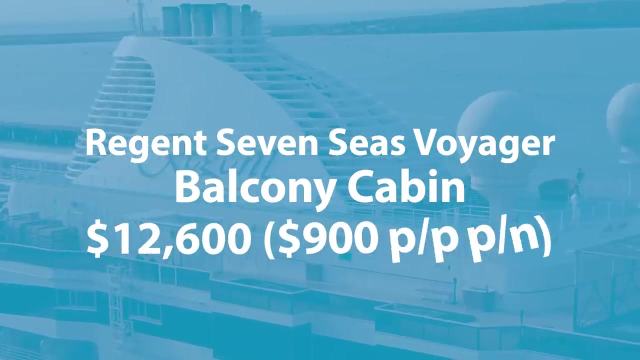 in their cheapest balcony cabin for $1,750.. $125 per person per night. Yes, book a very similar seven-night region seven seas voyager cruise in their cheapest balcony where one night would cost the same as that entire MSC seven-night cruise. That's a staggering $12,600. for two people for a week, or $900 per person per night. I asked Winnie to think about what she wants, those remaining lines that we've got left after that to add to her trip, as the ports and places are largely going to be the same. Does she want a deep immersion into Mediterranean history and 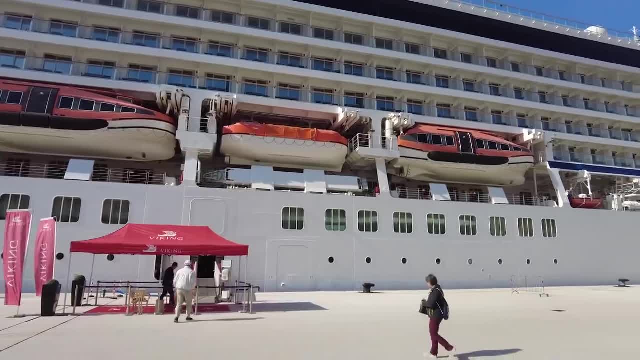 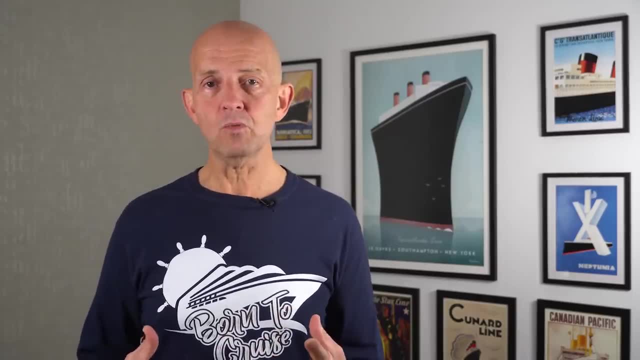 culture, for example. Then I would suggest she looks at lines like Viking, which have multiple daily lectures with an onboard resident historian. That may be best. Or perhaps does she want lots of late-night partying, big glitzy theatre shows, a really relaxed dress code. Then maybe MSC. 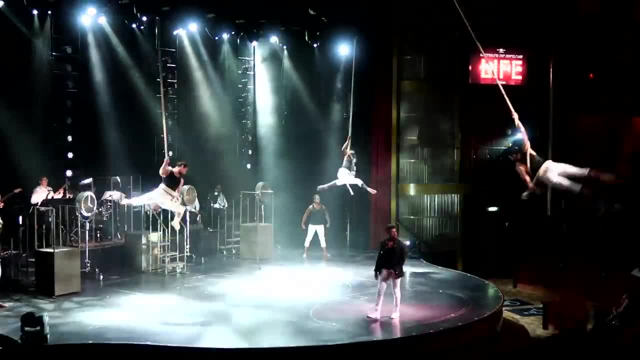 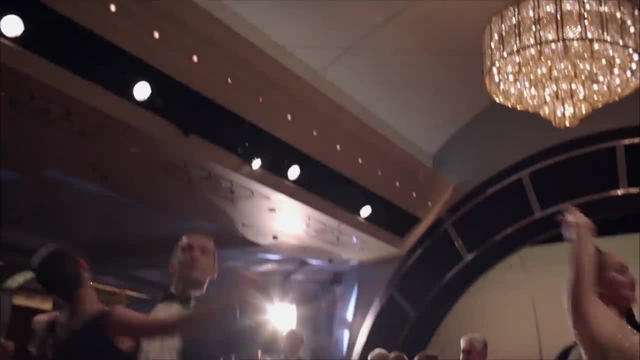 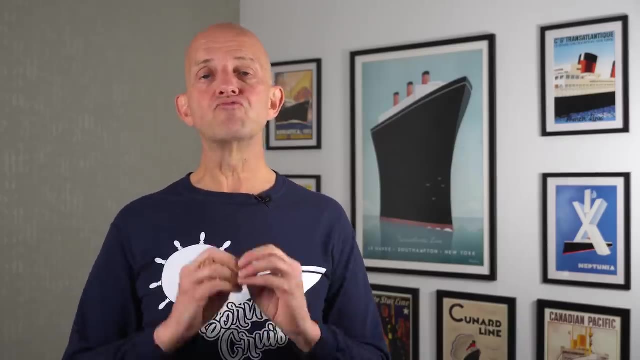 Norwegian Cruise Lines, Carnival or Royal Caribbean, for example, would be best. Or perhaps does she want a more familiar British experience with dressy, formal nights and live orchestra ballroom dancing? Then perhaps Cunard is going to be the one for her cruise, To avoid the trap of going on the 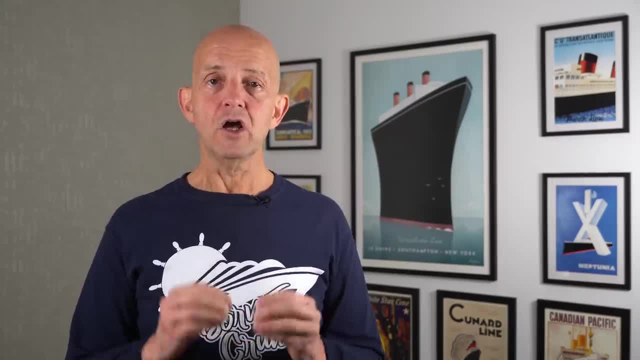 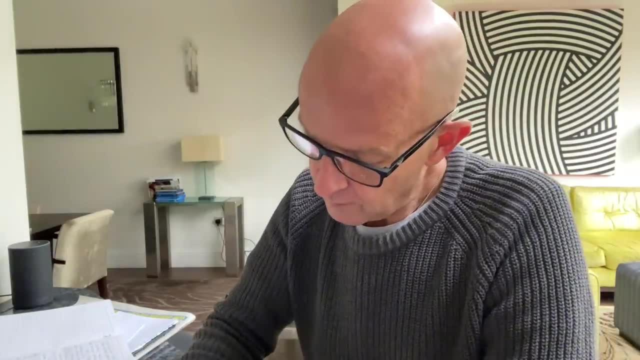 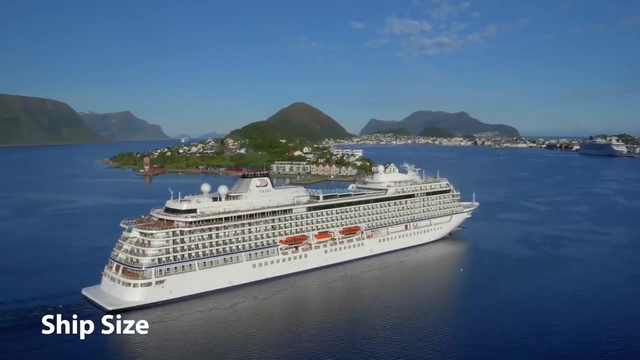 wrong cruise line and getting the most from her budget. Winnie agreed to draw up a list of what she really wanted from the ship and the line. Ship size, of course, is a valid consideration that she should have. Winnie had said that she thought a mid-sized ship because she heard there. would be less busy and have fewer queues, but more because she'd heard they would go to more interesting ports In the Mediterranean. the size of the ship is less critical in terms of what ports they call on than some other regions in the world. Definitely smaller ships can go into more. 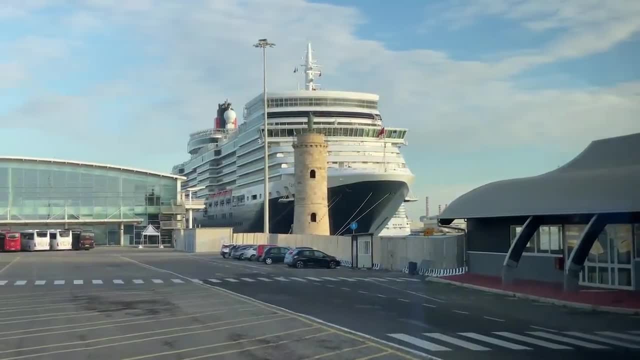 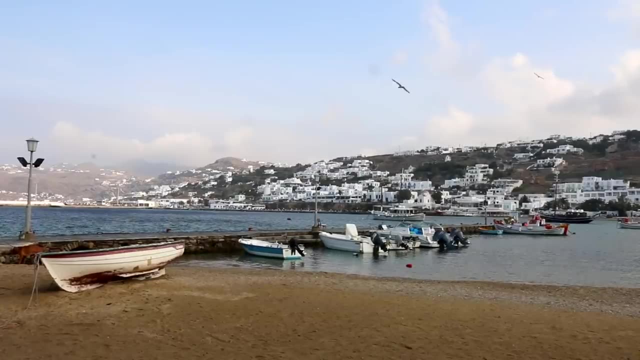 out-of-the-way ports, but that really applies much more in Greek Island itineraries than it does in the Western and Eastern Mediterranean. It's not as significant on those two itineraries. On these, most of the cruise ports tend to be used by all. 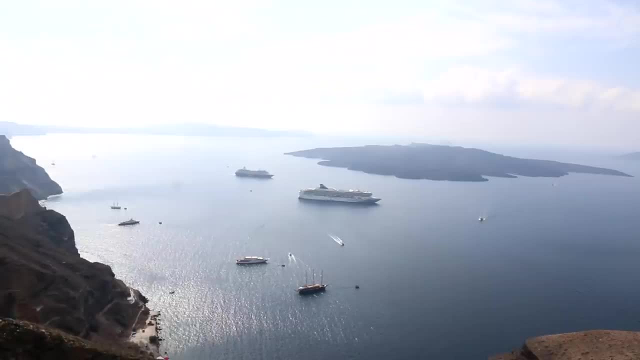 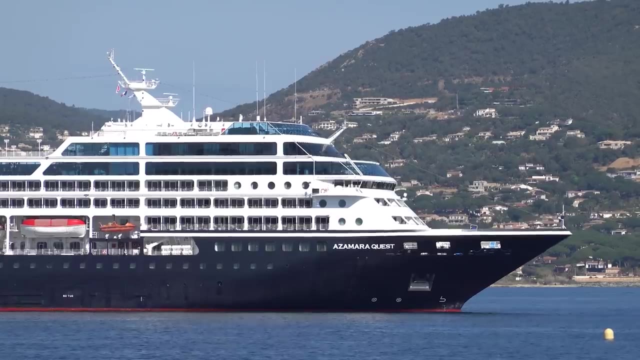 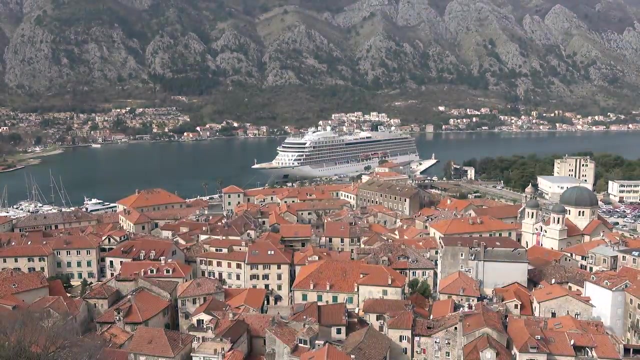 both big and small ships. So I suggested that she focus much more on the experience she wanted rather than the ship size alone. The next error Winnie almost fell into- but I think she got it right in many ways by chance- was that she was looking at a balcony cabin When he said online. 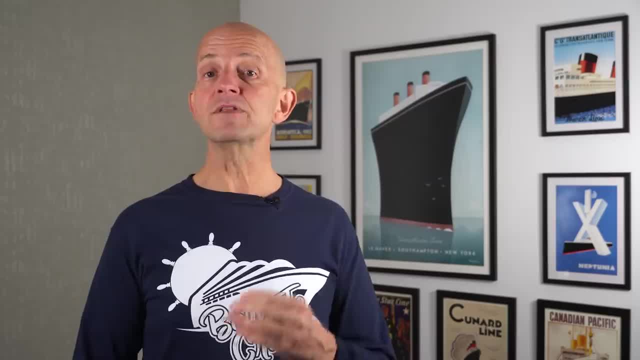 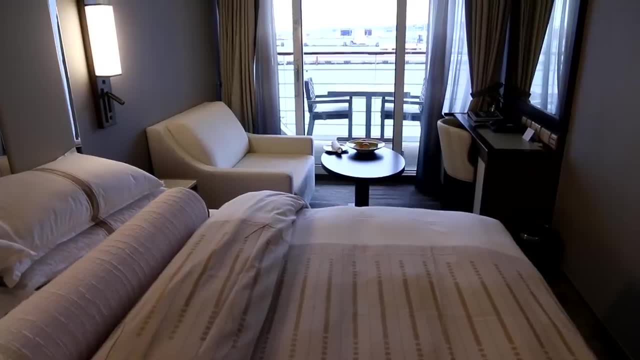 people were recommending to her that she take a balcony cabin because of the scenery to see while she was sailing in the Mediterranean. I don't think that is true. First of all, she's going to be sailing at night and then she's going to be way out at sea, and the only time that. she'll be close enough to view scenery is at sail in and sail out, both of which she may want to be out on deck for. I told her to choose a balcony over an inside or ocean view cabin only if she rated the upside and the experience worth the extra cost. I always choose a balcony when cruising. 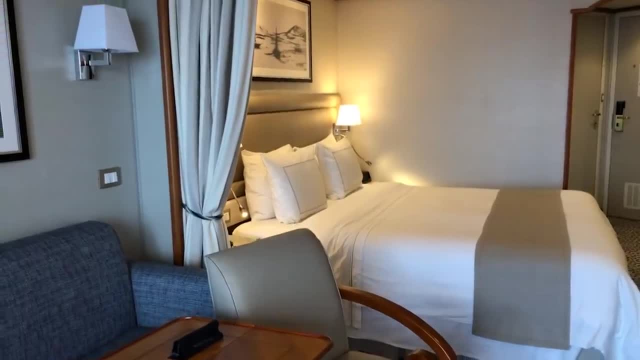 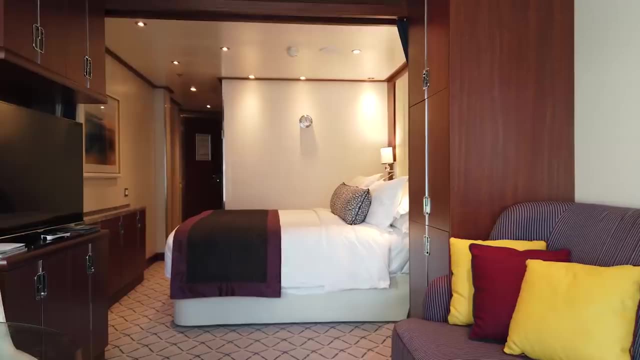 in the Mediterranean or pretty much anywhere as I like, being able to step out into the fresh air, sit there in the evenings when sailing out, and for the floor, two wall windows and all the extra light I pointed out on her cruise. she will.